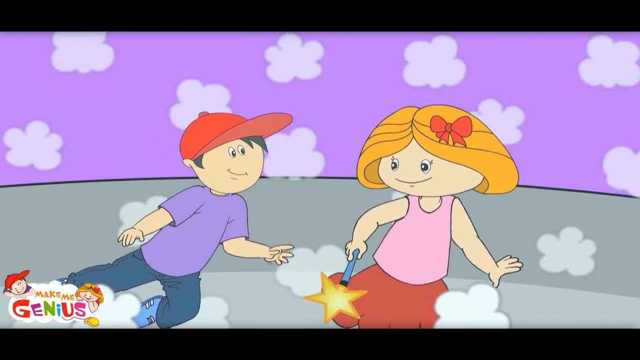 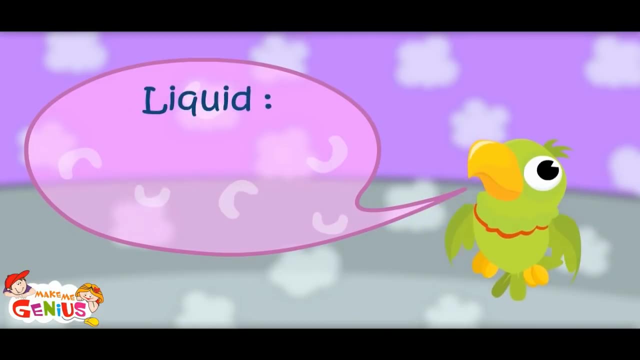 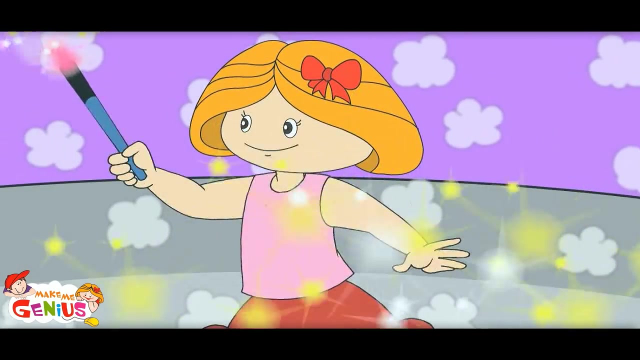 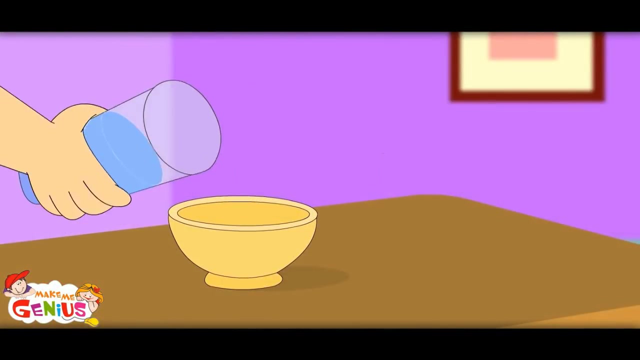 So they can go in any container and would take that container's shape. Hmm, Hey, Hey, Liquid molecules are apart and they take container's shape. Let's see how liquid changes shape. See, I was right, You put liquid in any container and it would take that shape, right? 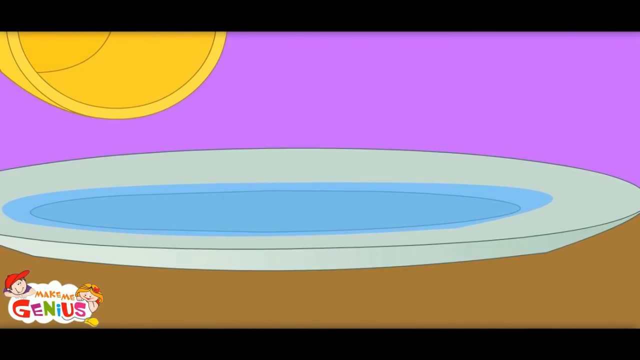 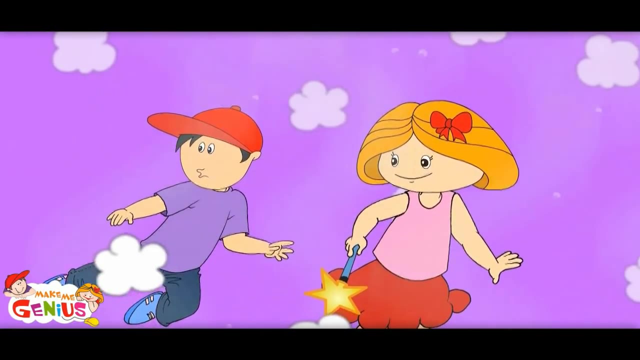 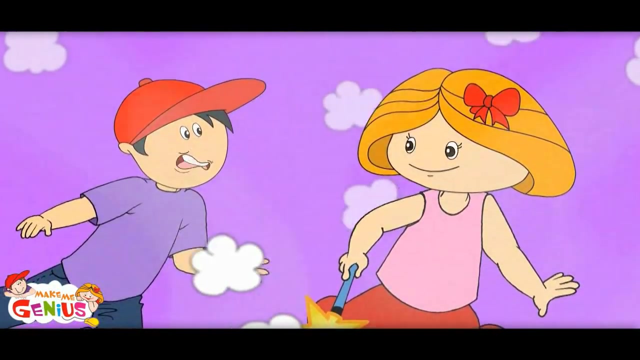 Yes, You are right, genius boy. Okay, let's enter the gas now. Aha, Here molecules are apart from each other, And see how fast they are moving. That is why they don't have a shape. Ah, Ah, Yes. 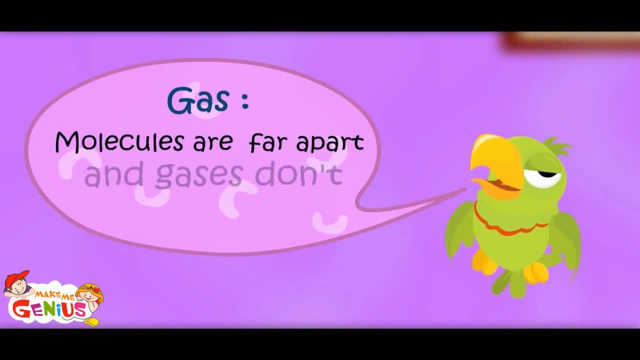 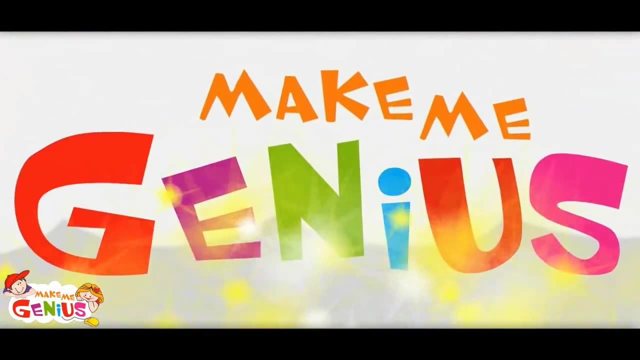 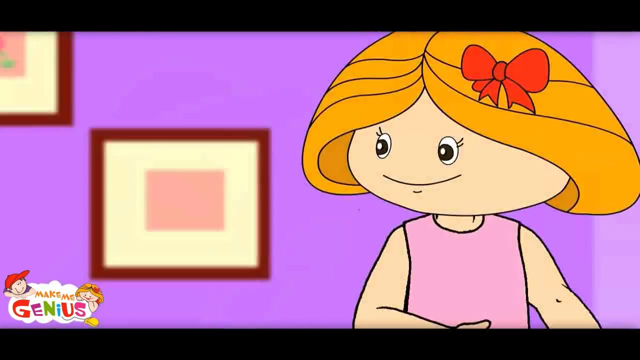 Molecules are far apart and gases don't have a shape. Let's again see all forms of matter. So this is solid, Yes. That is why it has a definite shape In your hands. water is in liquid form, Yes, And it takes the shape of the container. 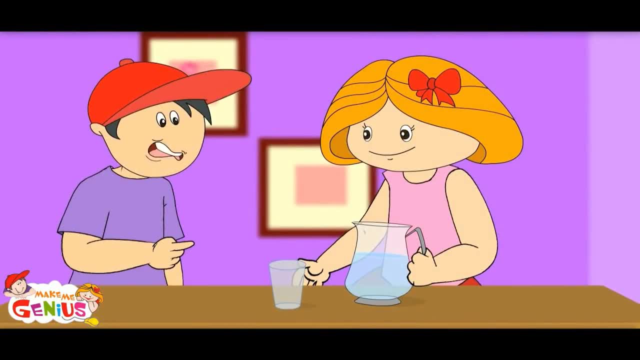 Like if I pour it in the glass, it would take the shape of the glass. Let's see again how molecules move in solids, liquids and gases. Yes, And it takes the shape of the container. Like if I pour it in the glass, it would take the shape of the glass. 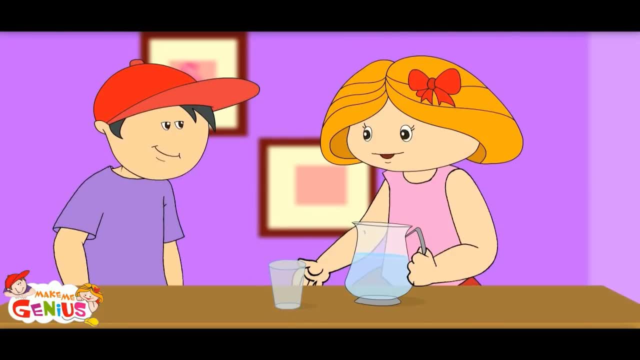 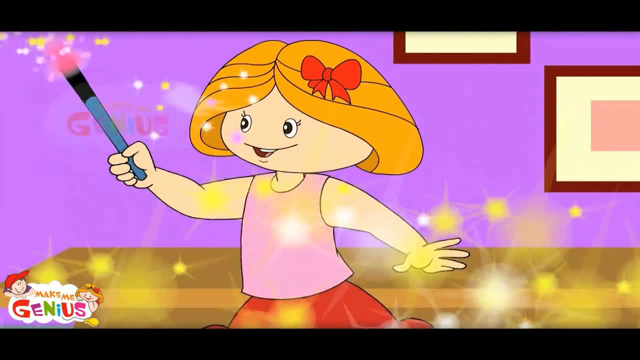 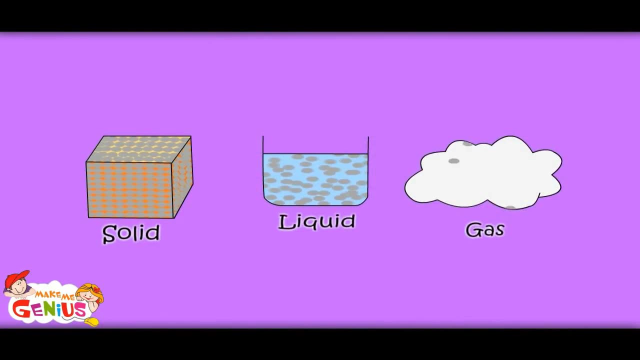 Like if I pour it in the glass, it would take the shape of the glass. Let's see again how molecules move in solids, liquids and gases, how molecules move in solids, liquids and gasses. Oh, now I can tell. 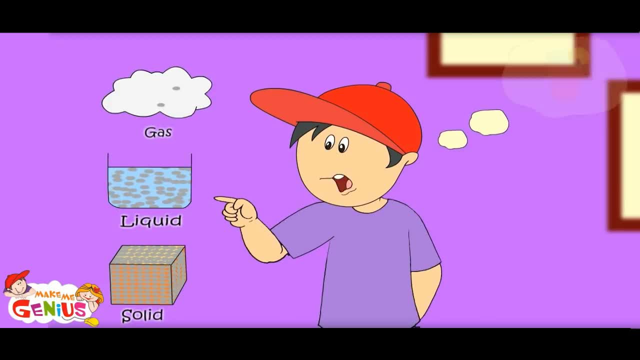 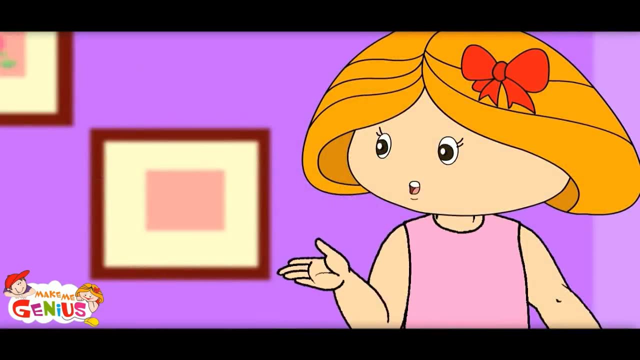 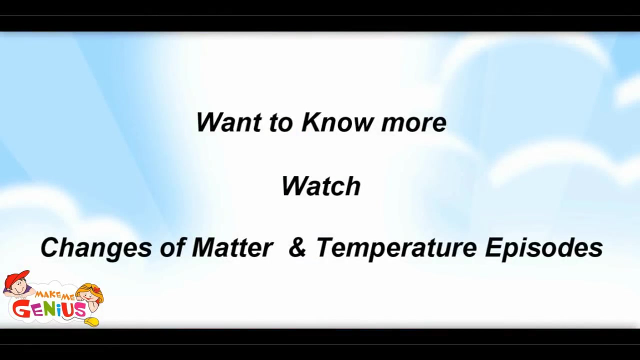 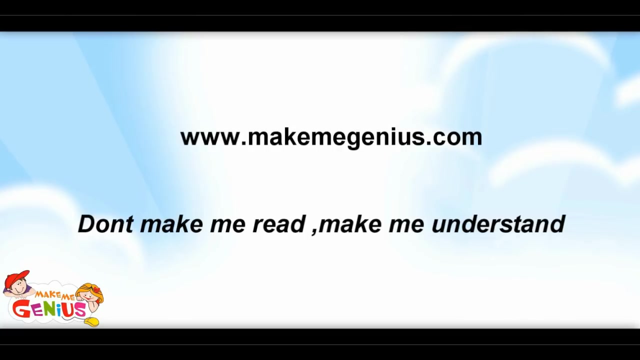 This is solid like spoon and it is liquid like juice And this is gas, like in a balloon. Yes, you are right. Let me note down all these things. Thank you for watching.